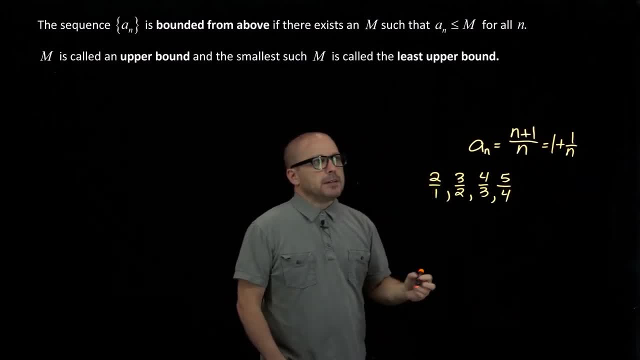 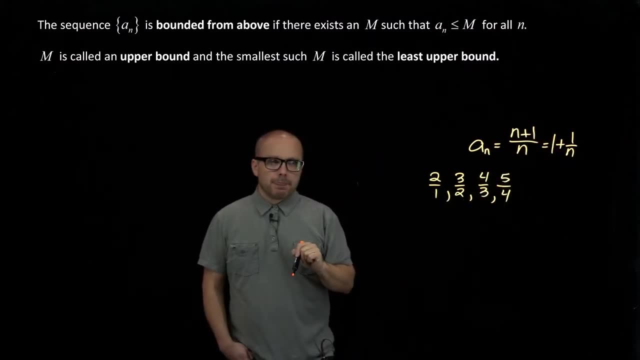 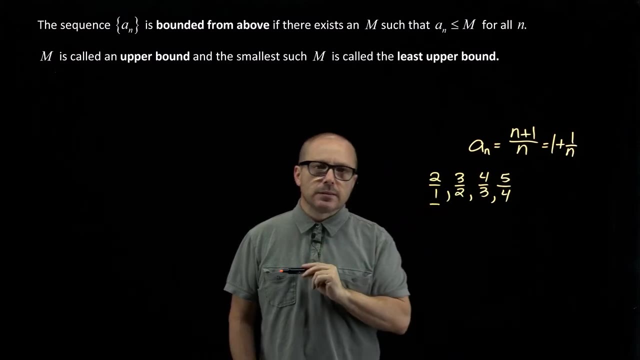 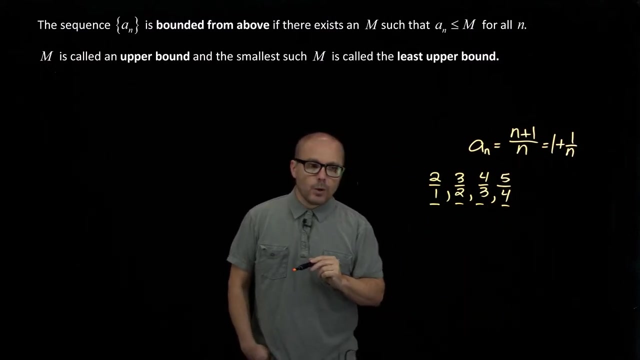 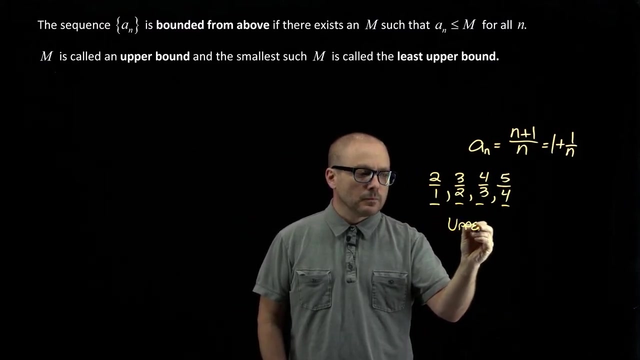 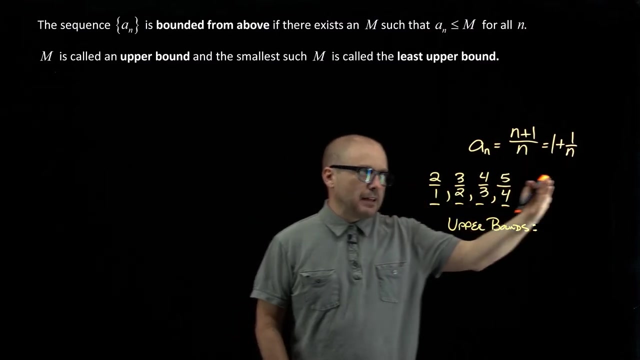 out at infinity is: it's 1 plus a little bit And that little bit's going to 0.. So this sequence is bounded above. The first term in that sequence is 2.. And every term after that is less than 2.. So we could say: for an upper bound, 2 works. 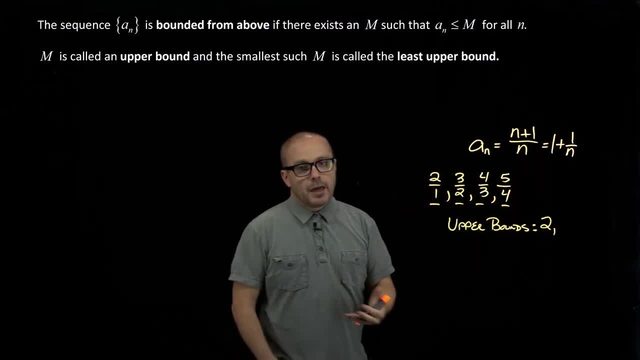 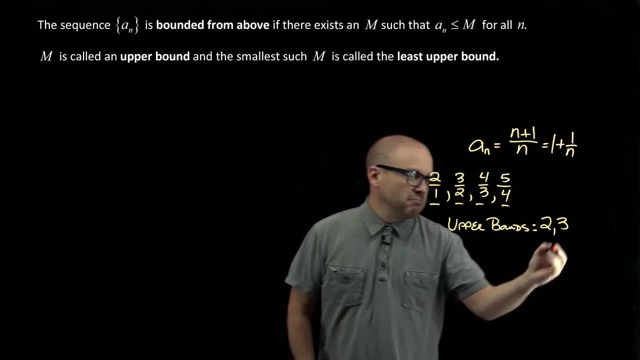 All numbers in that sequence are less than or equal to 2.. But really any number than bigger than 2 is an upper bound. If all the terms are less than or equal to 3,- excuse me, 2,, then they're also less than 3.. 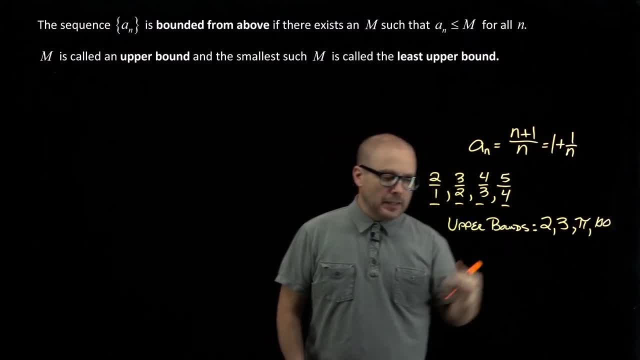 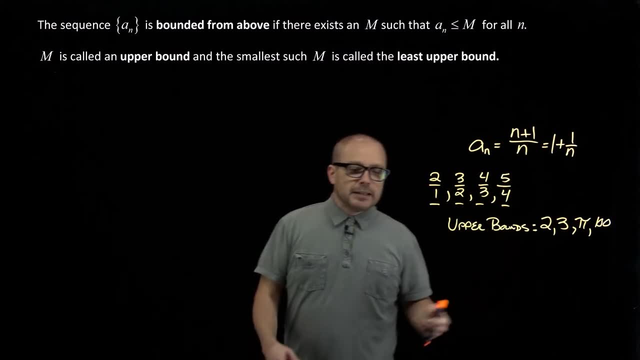 or pi or 100, any number you want to put there. So there's many, many upper bounds to this sequence. The key is that there is one, And then this last definition here is the least upper bound, So that would be the smallest number. that is still. 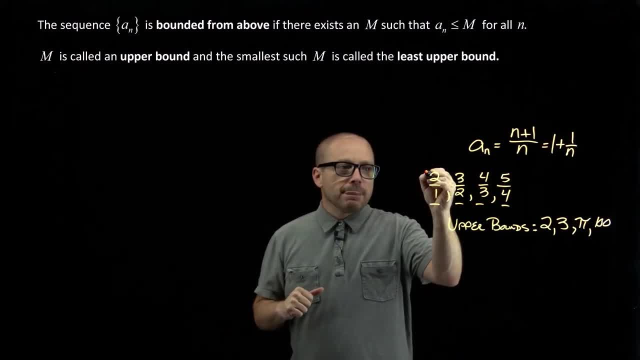 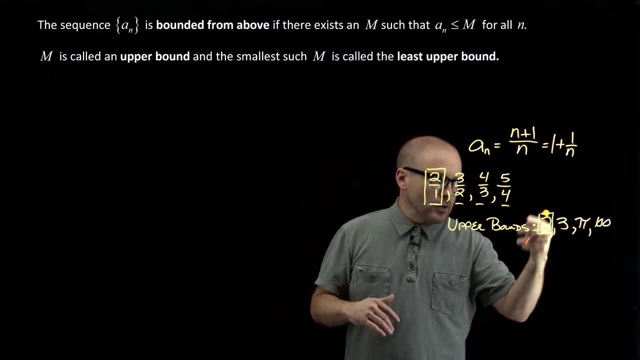 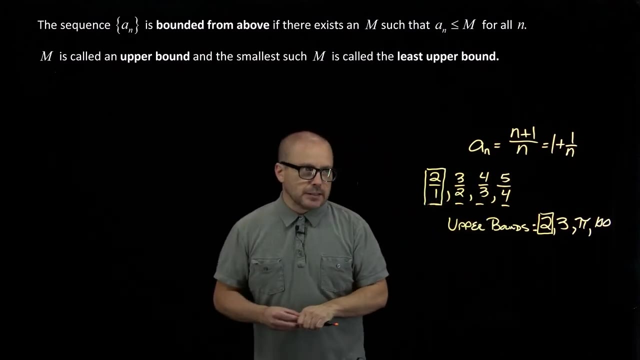 an upper bound on this sequence And that's this guy. I can't go any smaller than 2.. So these are all upper bounds, but 2 is the least upper bound. Any number I try and pick smaller than 2, all the terms in this list are not less than that. 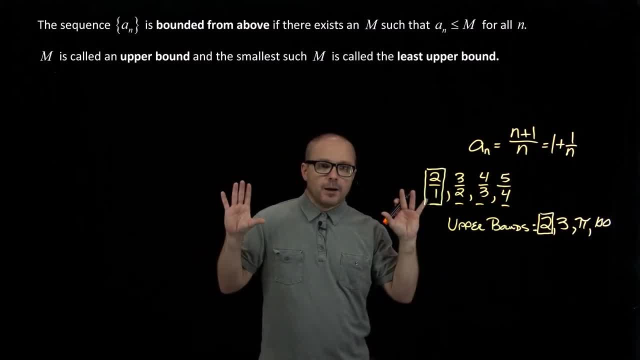 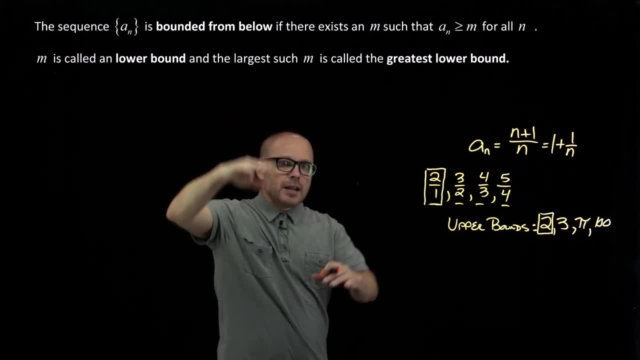 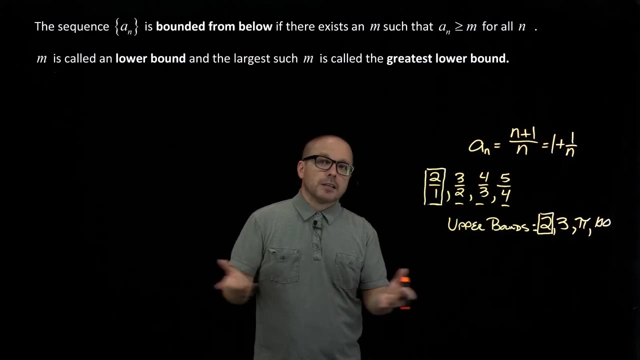 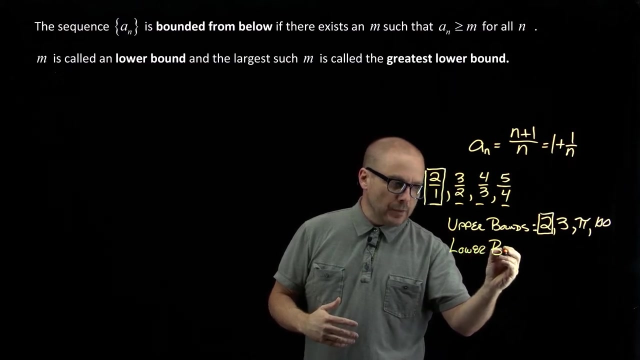 OK, so now let's look at the reverse side, being bounded below, So just have the flipped kind of definition. Now, if you could find a number that all values in the sequence are bigger, Then that's a lower bound, And so, for example, this sequence has many lower bounds. 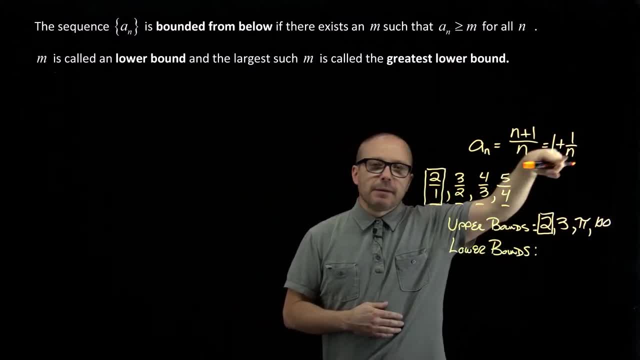 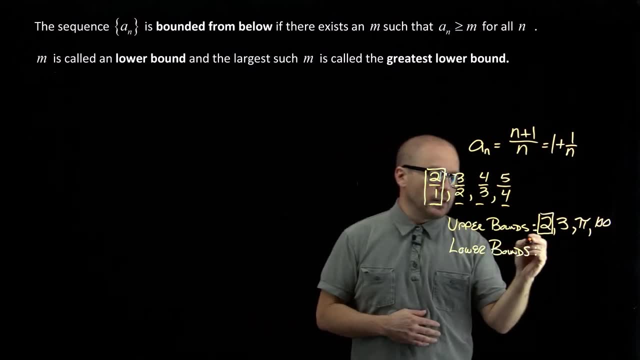 First of all, we know that what's happening here. We know that the limit out of infinity is 1.. These are all bigger than 1, but they're heading down, getting closer and closer and closer to 1.. So 1 works. 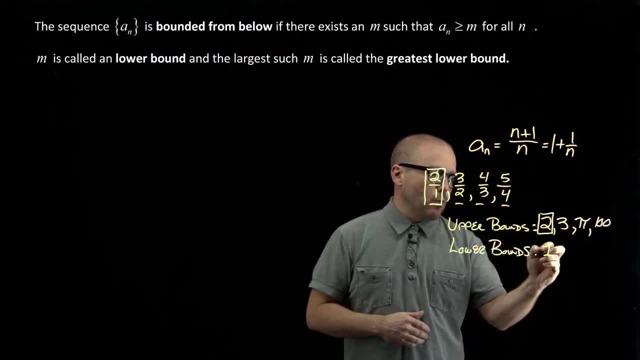 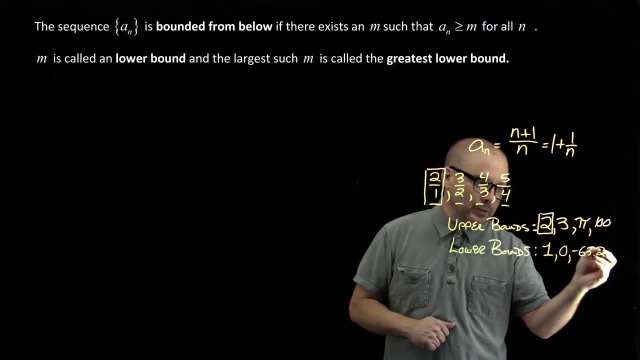 It's never going to be less than 1.. But just like upper bounds, if 1 works, anything smaller than 1 works. 0 would be a lower bound. Negative 63.2 is a lower bound- Any number less than 1,. all those terms are bigger than. 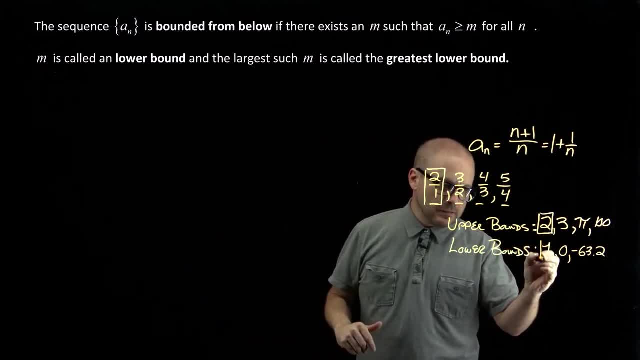 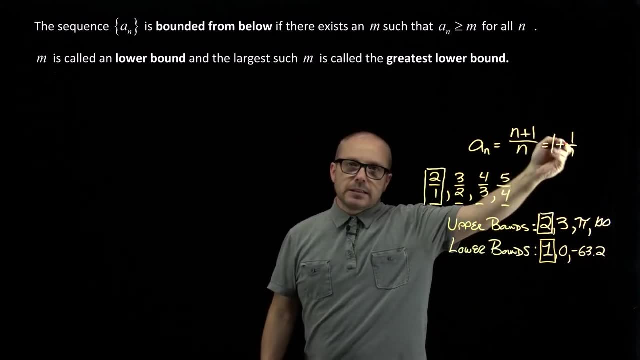 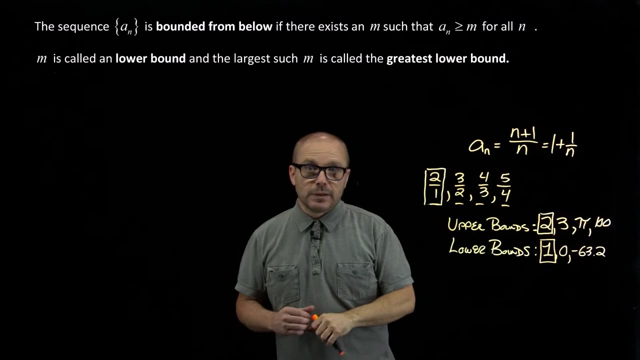 But the greatest lower bound is this guy. I can't pick any number bigger than 1, because eventually this sequence would be less. It's going to be less than that: 1.0000001,. well, if you go out far enough in this sequence. 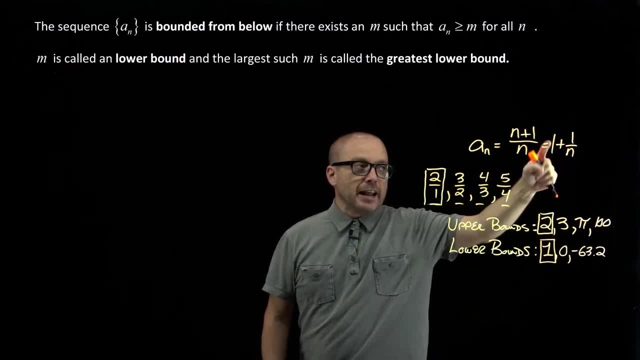 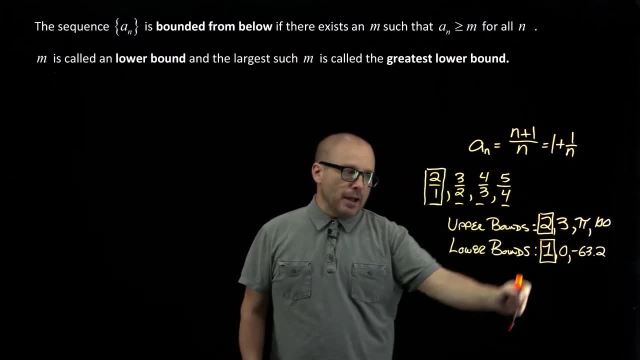 you'll be less than that because this thing's decreasing down and heading closer and closer and closer to 1.. So we've got all kinds of upper bounds- 2 is the least upper bound- All kinds of lower bounds- 1 is the greatest lower bound. 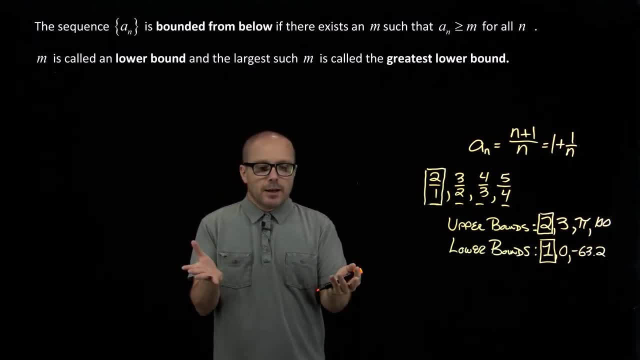 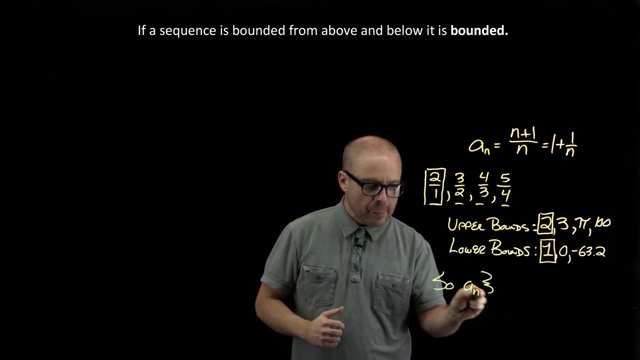 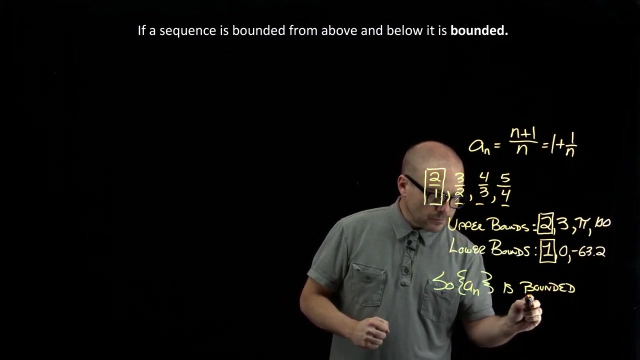 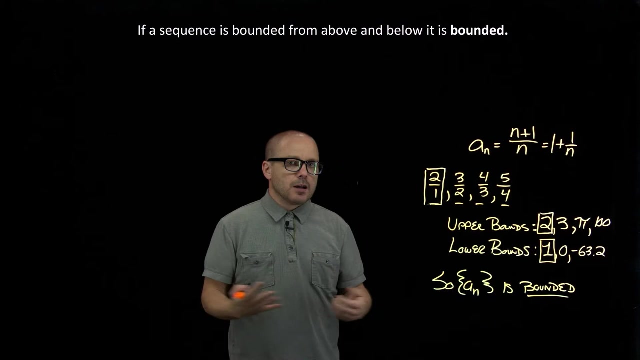 And then this sequence, because it's bounded both above and below. we say just generically that this is a bounded sequence, So our sequence is bounded. So this is some nice terminology to have, So we can talk about things being bounded above, bounded below. 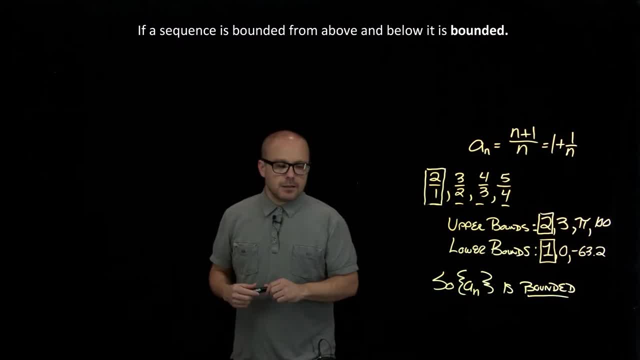 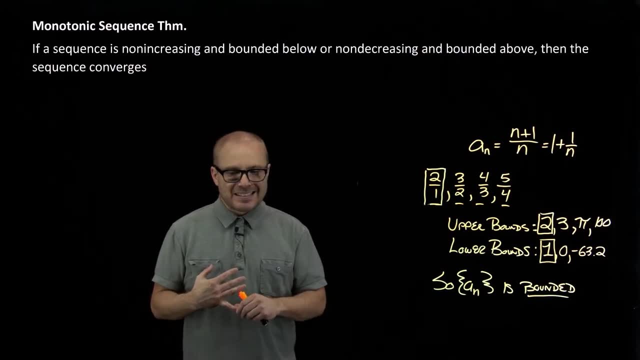 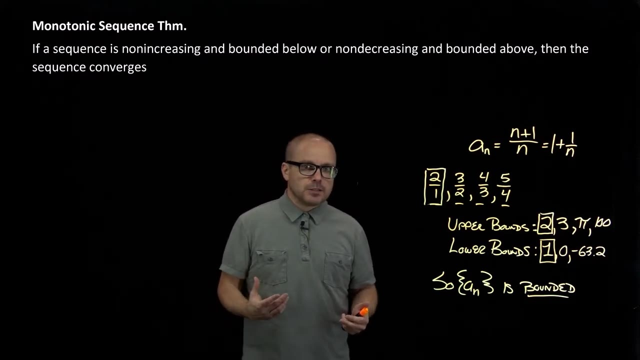 And now we know what we mean. So this sort of leads to a theorem that I want to talk about now, And that is the monotonic sequence theorem. So we've used the term monotonic in Calc 1.. It still means the same thing for sequences. 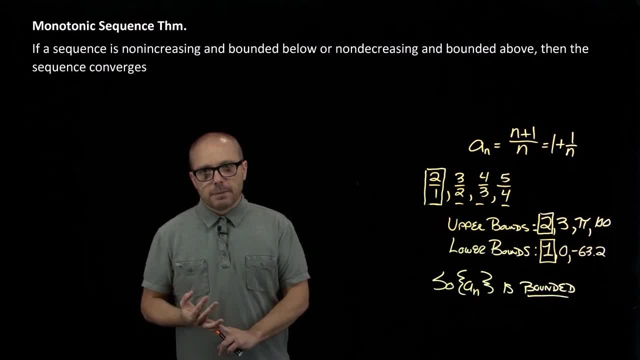 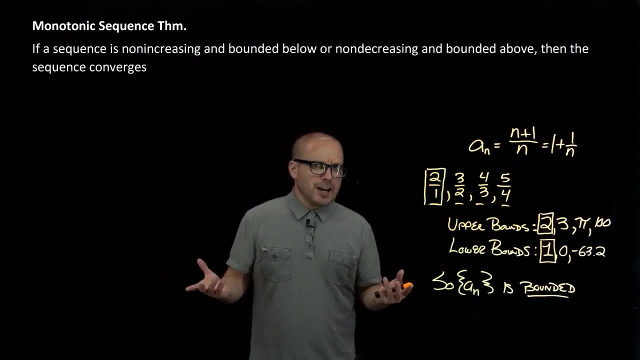 It means non-increasing or non-decreasing, And remember the first time you saw those terms may have been confusing, right? Because why do we call it non-increasing? Why don't we just call it decreasing, Or why do we call it non-decreasing? 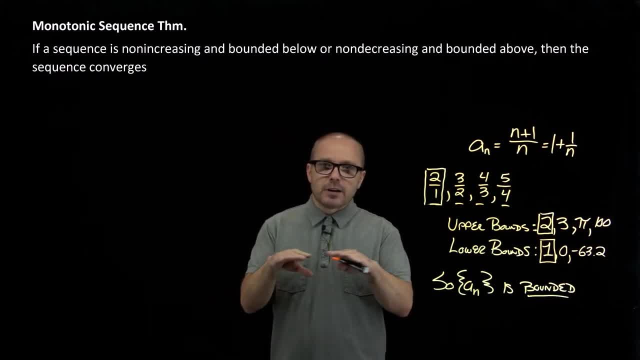 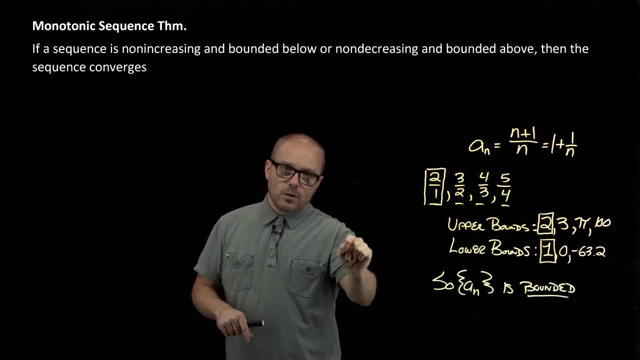 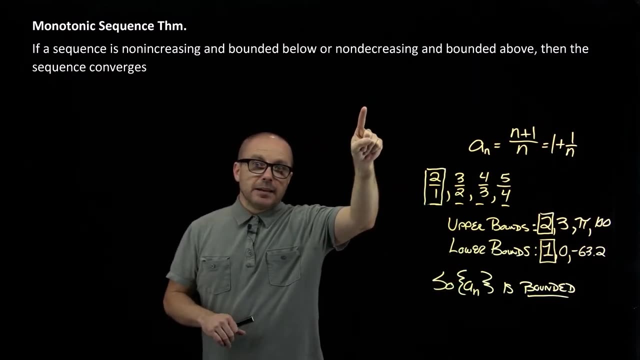 Why don't we just call it increasing? Well, it's because we want to allow for constancy as well. So non-increasing means that the sequence is always going down or staying constant For a while. it could do both. Non-decreasing means doing anything but decreasing. 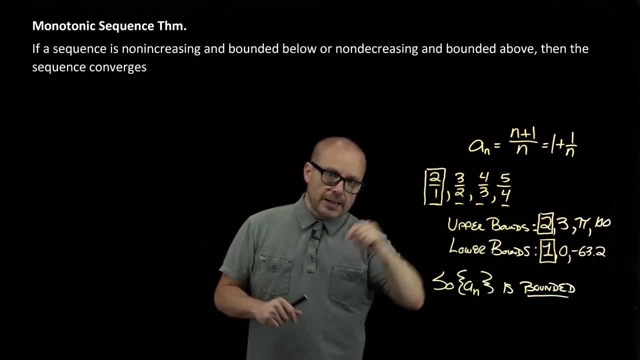 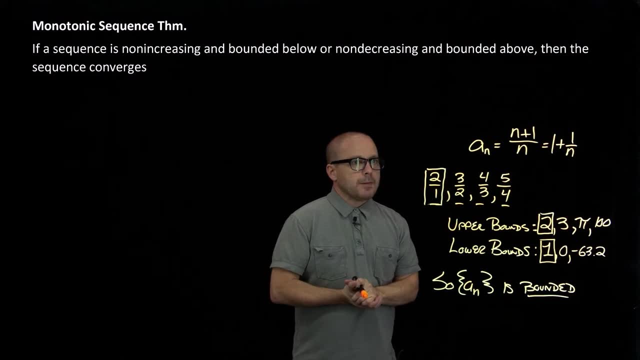 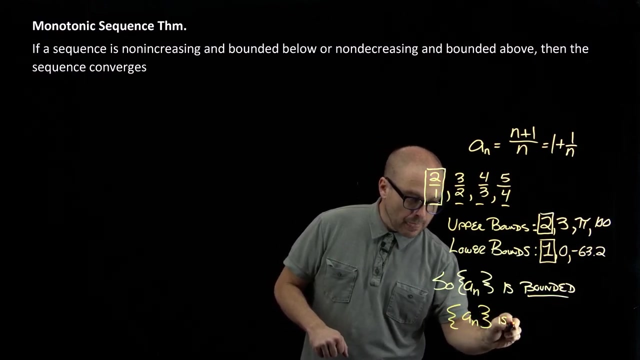 So it could go up or it could be constant, but it can't be going down. So, for example, this sequence- These guys are getting smaller and smaller and smaller and smaller- It is non-increasing, right. So our sequence is non-increasing. 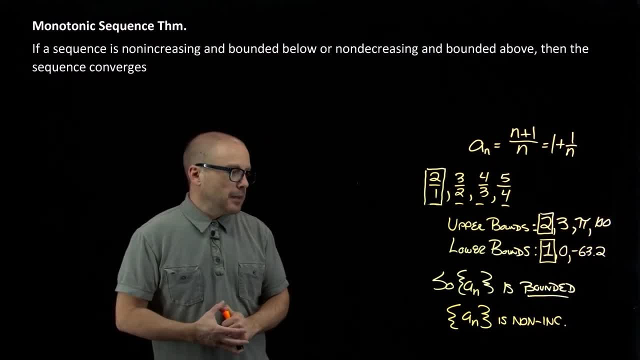 So what we have is a bounded sequence that is monotonic Right. Monotonic just means you're going to have a sequence Right. Monotonic just means you're going to have a sequence Right. So you're either non-increasing or non-decreasing. 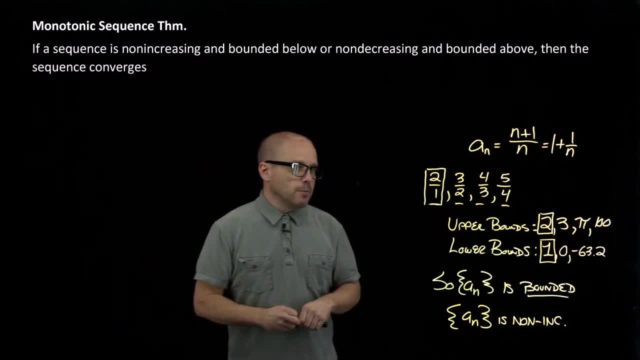 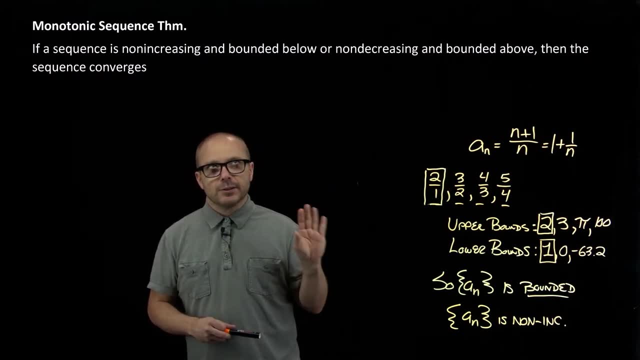 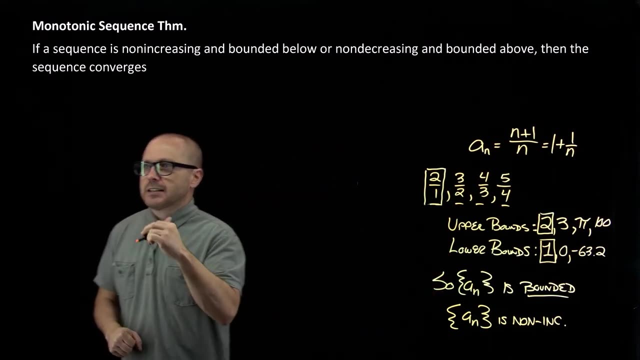 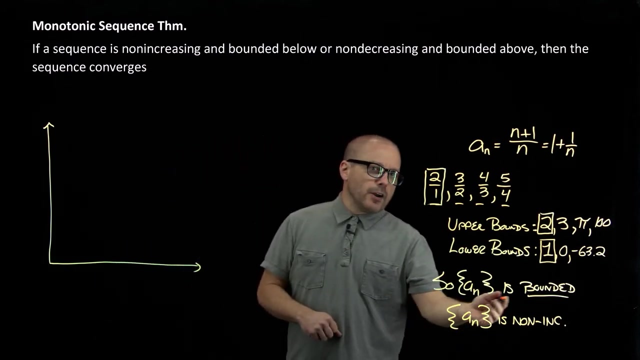 If you have that sort of behavior either direction, you're considered monotonic. Well, the theorem says that if you combine those two things, the sequence must converge. And let's just think about that graphically for a second: We are non-increasing, right. 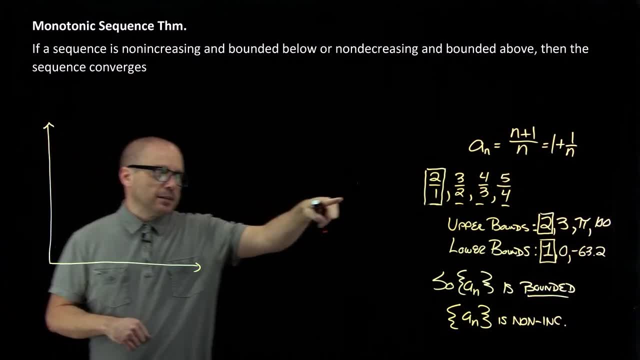 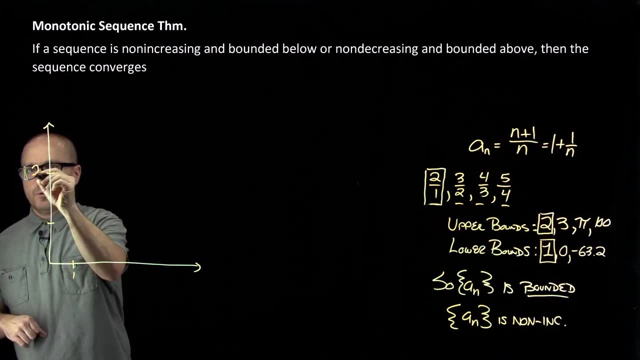 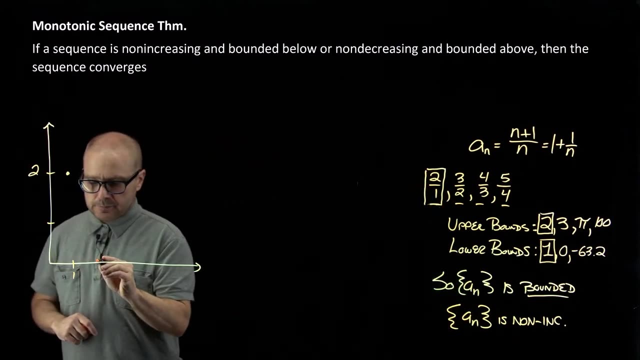 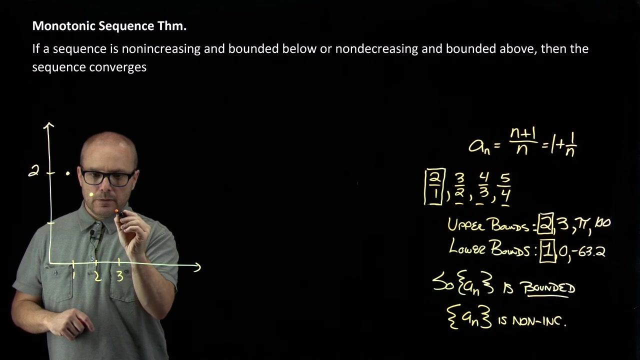 So just in general, In general, if I draw something, maybe not necessarily. well, yeah, we'll go ahead and draw our terms. The first one was 2, right. The next one is 1 and 1, 1⁄2, and then 1 and 1⁄3, and so on. 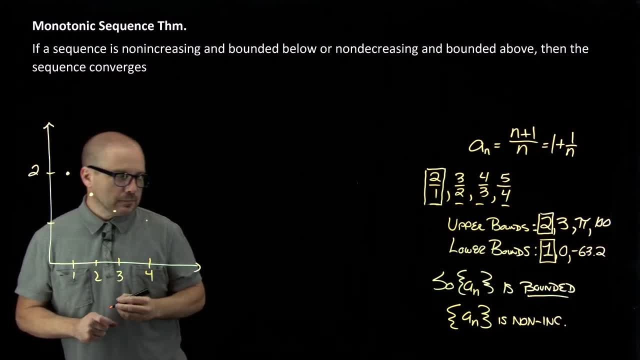 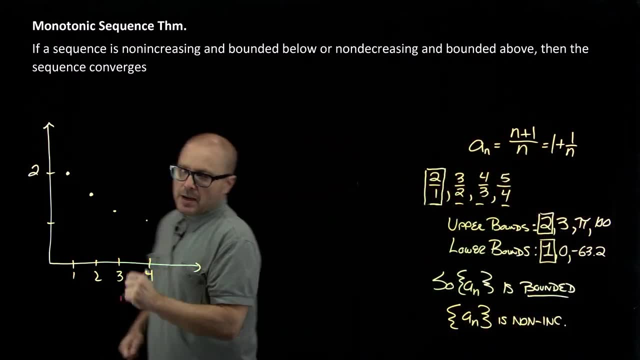 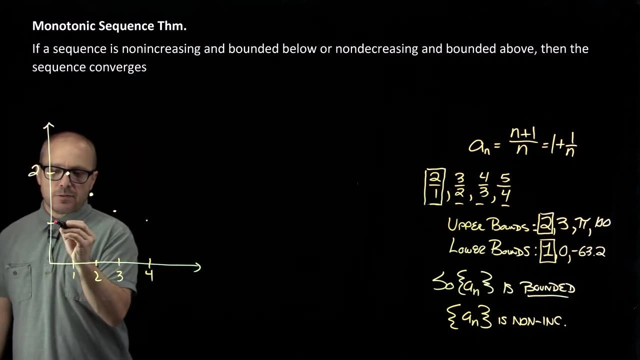 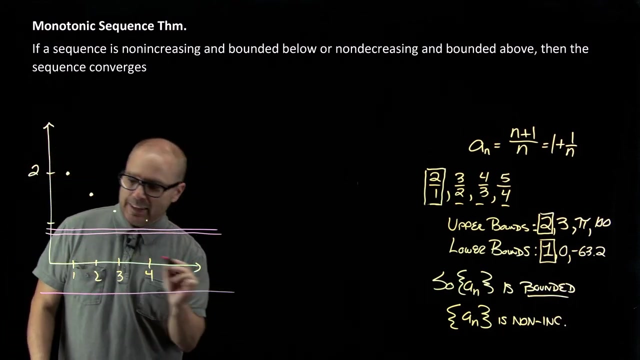 But it's bounded. So now I'm not going to necessarily draw that one, I'll just draw many. There's many lower bounds for this thing, right? Those dots never get lower than that. They never get lower than that. They never get lower than that. 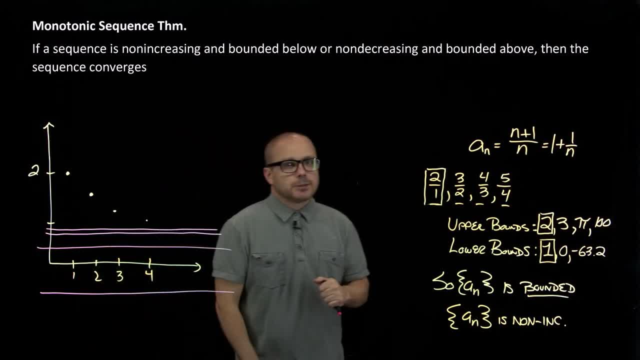 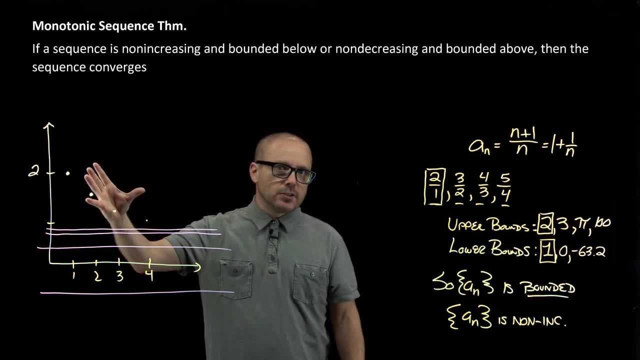 There's many lines I could draw here. These are all lower bounds on that sequence. But what's nice Is, even if I can't prove what this converges to, I know it has to converge And that's what the theorem is saying. 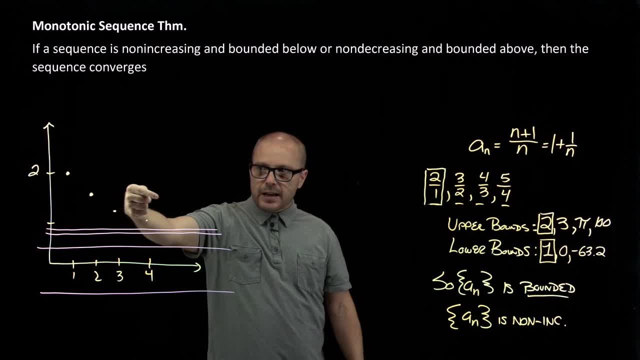 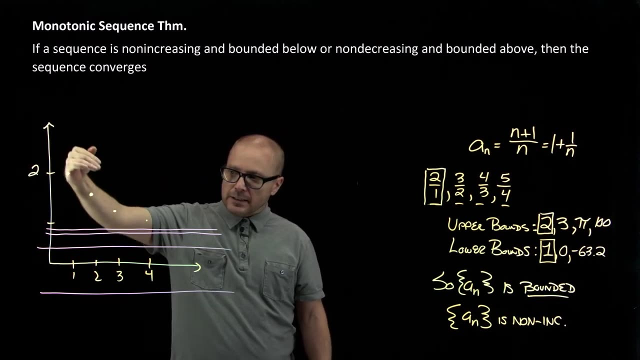 If you're going down or staying constant and you have a lower bound, you have to converge Because you can't go beyond that. But you can't turn around and go back up Because you're monotonically, in this case, non-increasing. 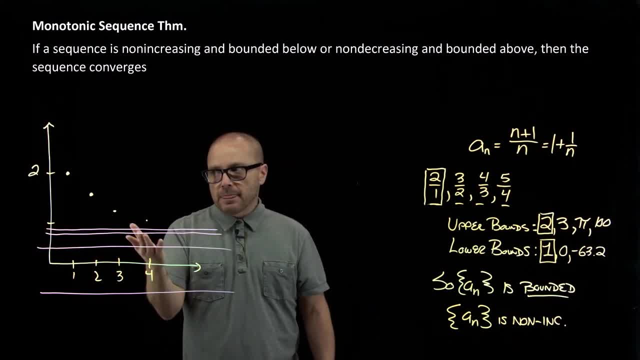 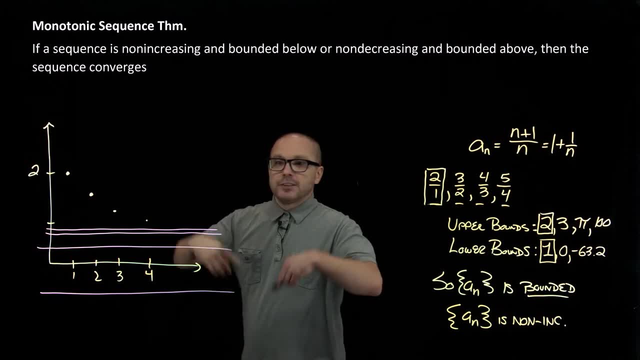 and bounded below. I'm going to converge. Now I'm not saying what I'm going to converge to, But it's good to know that that's a convergent sequence. Now the flip side. this covers both directions, right? 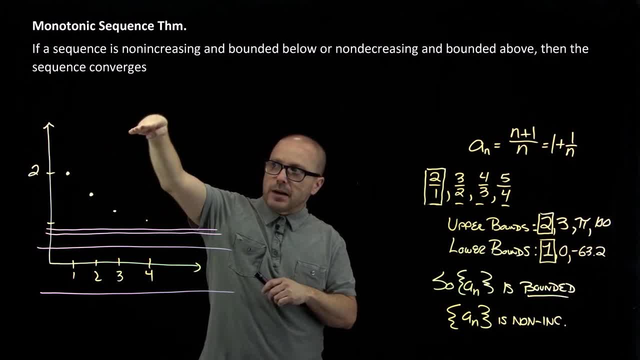 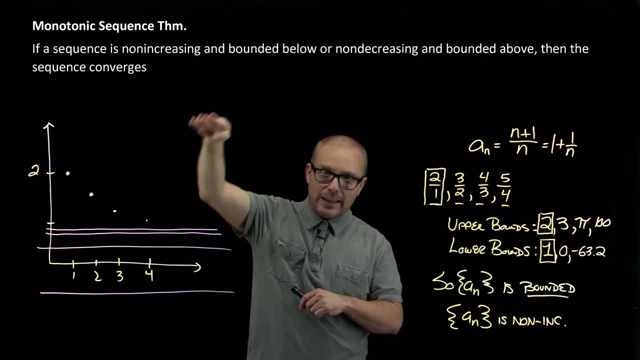 That could be non-decreasing. Well, if you're going up and up and up- possibly constant for a while, but up and up- and you have an upper bound, you have a ceiling that you can't cross and you're not allowed to turn around and go back down.